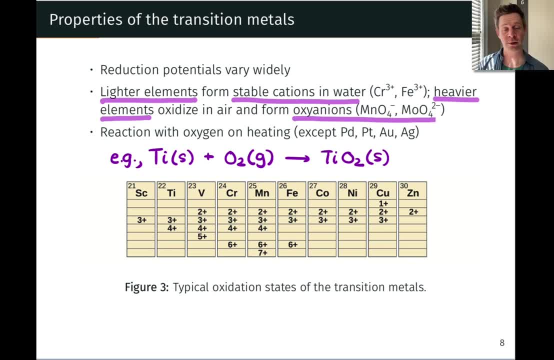 heating titanium metal in the presence of oxygen gas will lead to the production of titanium 4 oxide as a solid, And notice that this is an oxidation of the titanium metal, which is in zero oxidation state, to TiO2, in which titanium is in the plus 4 oxidation state. So this is just 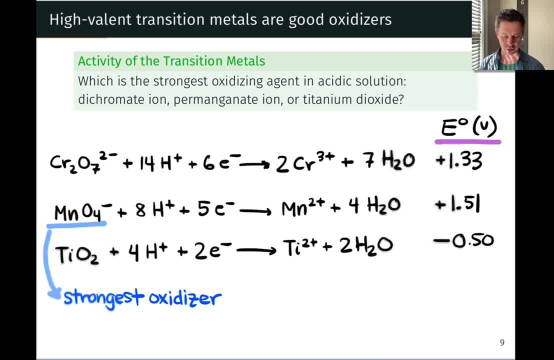 a general overview of the typical properties of the transition metals And I wanted to close this discussion of transition metals with a little bit of information about the transition metals. So let's take a look at some of the transition metal properties, with just a brief look at some. 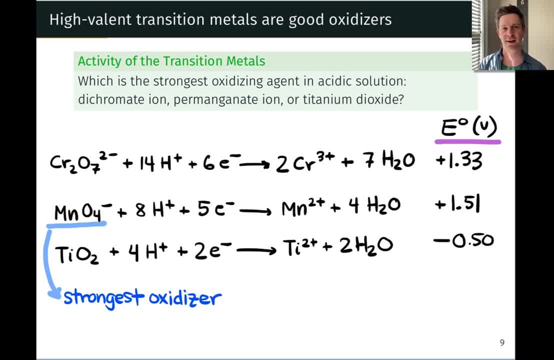 reduction potentials related to transition metal containing species, just to show that these can vary over quite a wide range depending on the nature of the transition metal. So the focus here is on dichromate permanganate. these are oxyanions containing chromium and manganese. 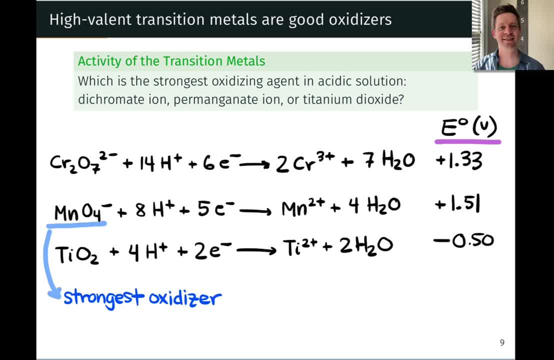 respectively, and titanium dioxide, which is an oxide of titanium, obviously with titanium in the plus 4 oxidation state. If you look at the reduction potentials for each of these species, you can see that both dichromate and permanganate are pretty good. 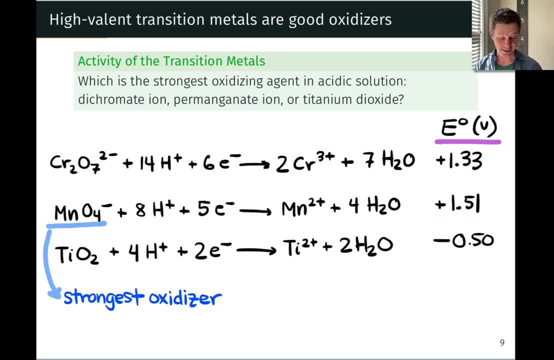 oxidizers with a positive reduction potential, indicating that they're readily reduced. They will readily pull electrons from a reducing agent and become reduced themselves, acting as oxidizers in the process, And permanganate is the strongest oxidizer on the list, with the most 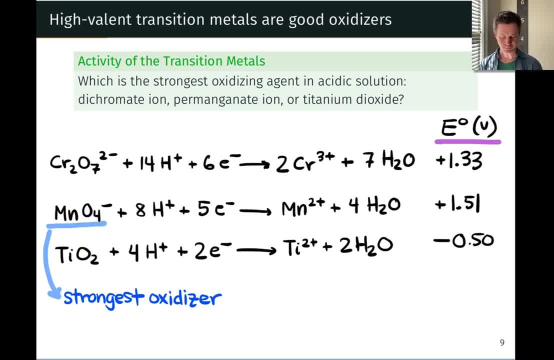 positive reduction potential for the permanganate anion. On the other side of the coin, TiO2 is not a very good oxidizer, despite the fact that it's a very good oxidizer. So if you look at the presence of oxygen in the compound, its reduction potential is only negative 0.5 volts, so a 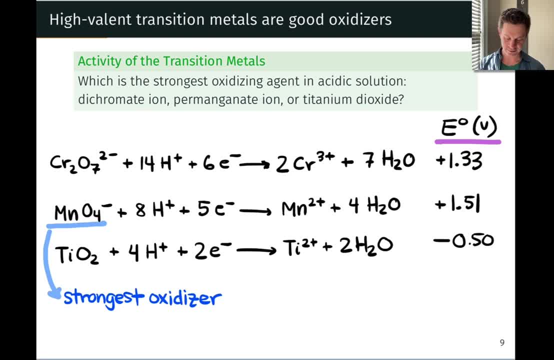 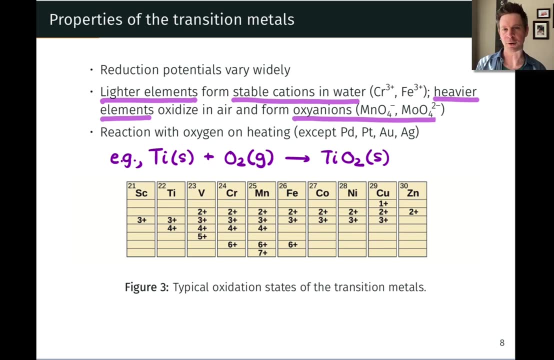 difference of about 1.8 volts from the pretty good oxidizer- sorry, about 2 volts- the really good oxidizer, permanganate, known for being a good oxidizer to TiO2, which is not known for being oxidizing really at all. To close this video, let's take another look at typical oxidation. 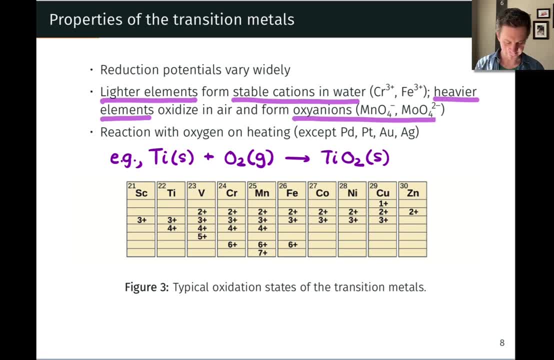 states accessible to the transition metals. This figure focuses on the transition metals and we're going to focus on that first row of the transition series, with the 3d subshell being filled, And one thing we can notice is, first of all, the plus 2 oxidation state is extremely common, starting at